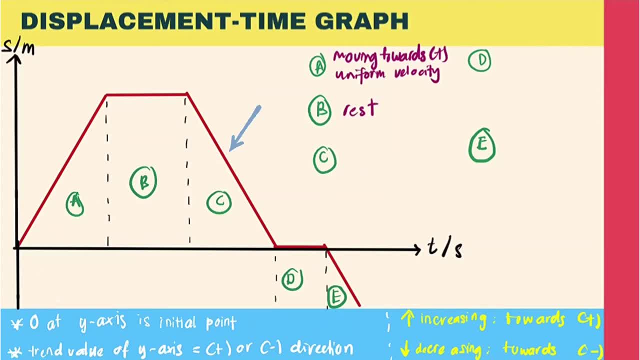 decreasing linearly all the way to point zero, which means at section C the object is moving towards the negative direction all the way to initial point. And at section D the graph is plotted straight across at point zero, which only means one thing: At section D the object is stationary or resting at the initial point. 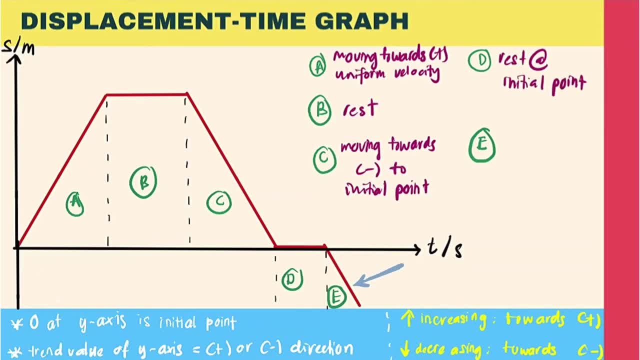 At section E, the graph is plotted decreasing linearly below the x-axis, which means that the object is moving towards the negative direction past the initial point. There's a few things to know that could help you understand the displacement time graph. First off, you need to know that the zero at a y-axis of a displacement time graph is the initial. 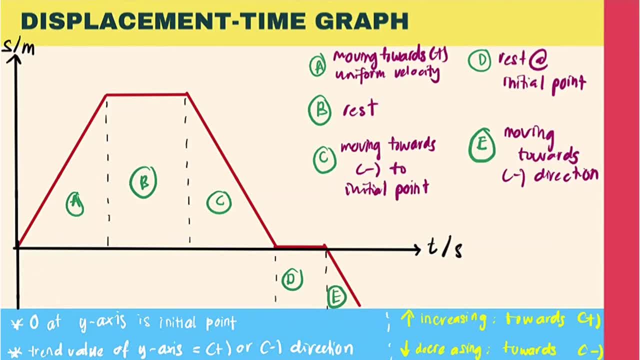 point. So, just like at section D here, since it is plotted straight across at point zero, this means that during this time the object is at the initial point. In order to know the direction of motion of the object, just look at the trap value of y-axis. 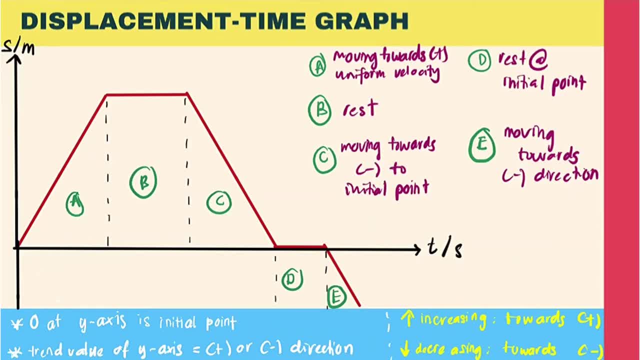 At section A, the value of y-axis is increasing, which means that the object is moving towards the positive direction. At section C, the y-axis value is decreasing, which means that the object is moving towards the negative direction. In order to help you understand this better, I will show you the motion that is represented by 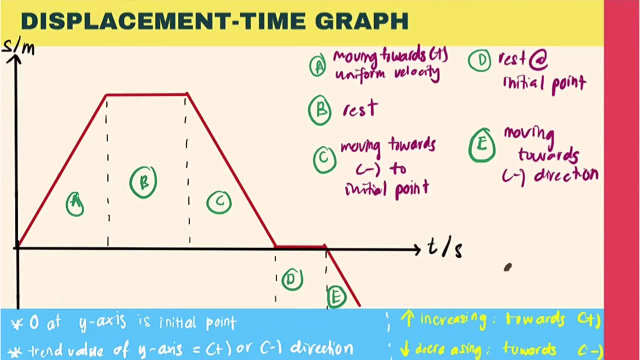 this graph. Let's say that the object here is this point right here For section A. the object moves towards the right, So this will be motion A, Then the object rests for a few seconds and that will be motion B, And then the object moves all the way back to the initial. 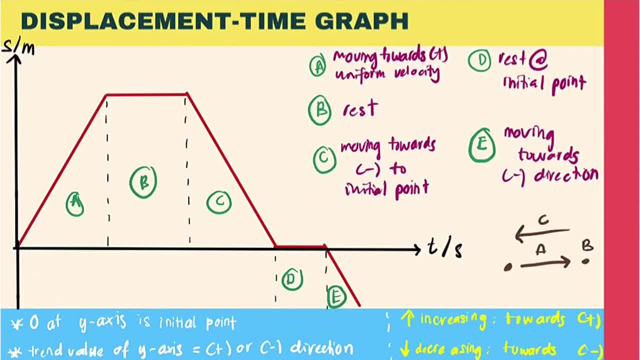 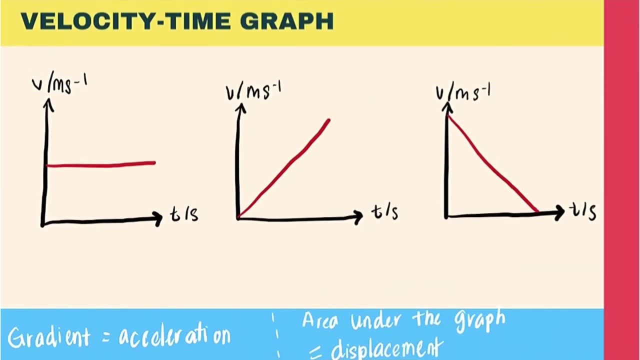 point towards the negative direction, So that will be motion C. Then the object rests at the initial point, So that will be motion D, And then the object moves towards the negative direction past the initial point, So that will be motion E. Next let's look at a velocity time graph. Velocity time graph records the velocity of 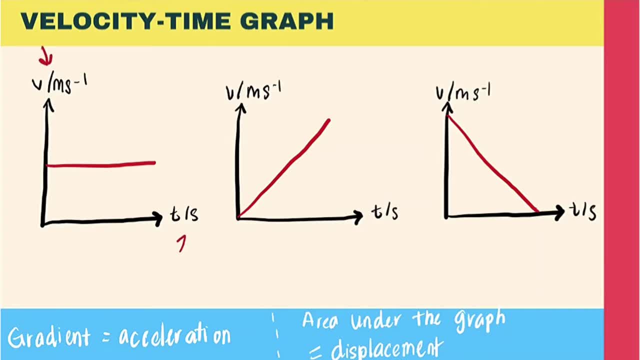 an object at the y-axis against time at the x-axis. Let's look at some basic trends of a velocity. If the graph is plotted straight across, just like number 1 here, this means that the object experiences a uniform velocity. So that would be zero acceleration If the graph is plotted. 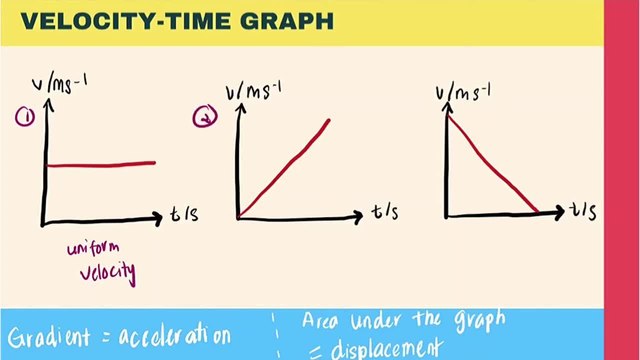 increasing linearly, just like number 2 here, this means that the object undergoes a uniform acceleration. Next, if the graph is plotted decreasing linearly, just like number 3 here, this means that the object is undergoing a uniformly decreasing velocity, or you might say as a uniform deceleration. 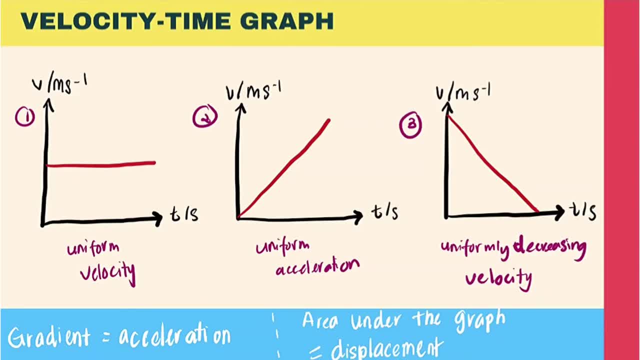 There's a few important things to note about a velocity time graph. First off, if you calculate the gradient of the velocity time graph, you will get the acceleration of an object. To find displacement of an object or distance travel, just calculate the gradient of the velocity time graph. 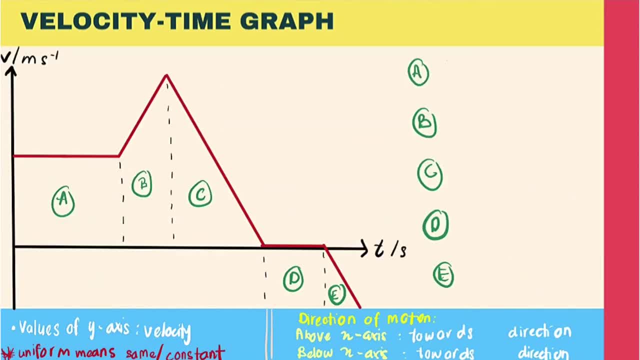 Now to end the video. you can revisitAngleRunning south coast traffic environment and do it a little further into the video so you can see the deff nicely. And now let's be accurate. So if the graph is a normal velocity time graph, Next, let's analyze a common velocity time graph, like the dimension I did earlier. As you can see, as you often do, as we've seen a lot in computers- it may be easy to interpret with a algebraic scale. For this reason, it's important to suppose that Guinness looked up the engineers'. algorithm to find theaste equation from the mathematical equation Even earlier. the calculator would be quite simple. but after reading the expectations things here, we can see that that couple of ones from each department еще anderen Mm, hmm, or at least 4 of 6 would sum up ourEM minimum velocity. 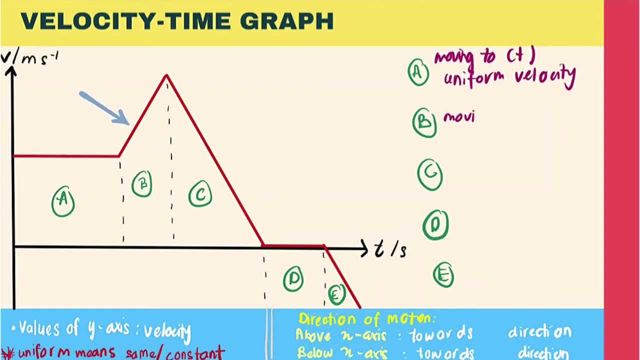 Next let's analyze a common velocity time graph. at section B, the object is moving still towards the right, but with uniform acceleration. At section C, the graph is plotted decreasing linearly all the way to point zero, which means that it is moving still towards the positive direction. however, the velocity is decreasing. 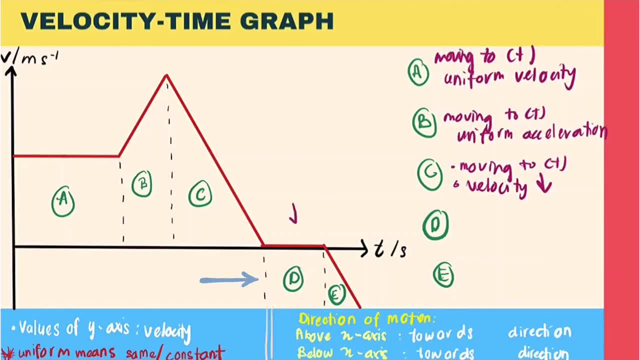 at section C. At section D: here the graph is plotted straight across at point zero, which means that the object is at rest, And at point E: here the graph is plotted decreasing linearly below the x-axis, which means that the object is moving towards the negative direction. however, 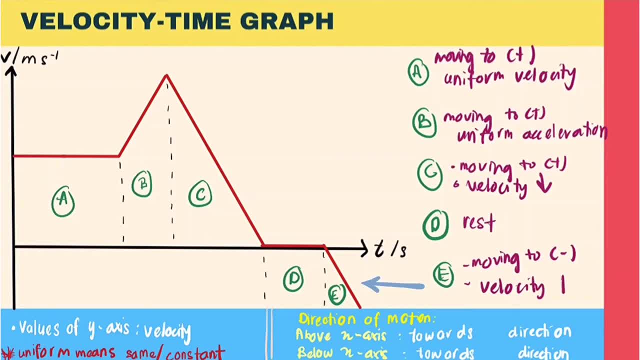 the velocity of the object still increases. It is very difficult to understand a velocity, then understand вполне easily at some point. so the graph is moving, declining If we calculate a time graph. So here's a few tips on how to understand this graph better. First off, 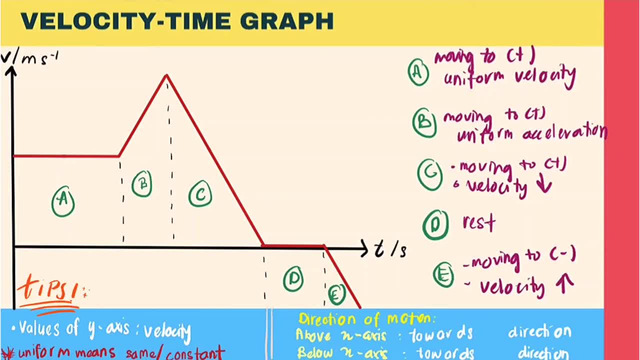 you need to know that the values of the y-axis of a velocity time graph corresponds to the velocity. For example, if we look at section A here, the value of y-axis at section A is the same, which means at section A the velocity is. 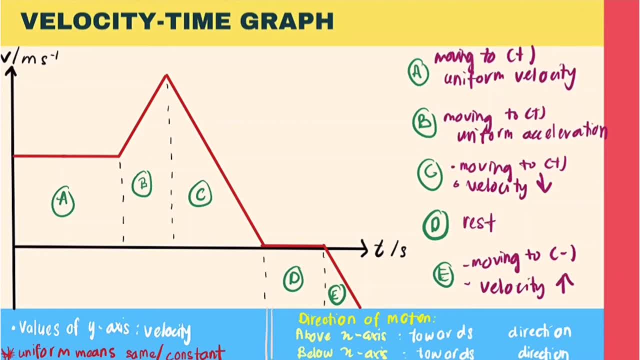 constant To know the direction of motion. you must know this. If the graph is plotted above the x-axis, just like A, B and C here, this means that the object is moving towards the positive direction. If the graph is plotted below the x-axis, 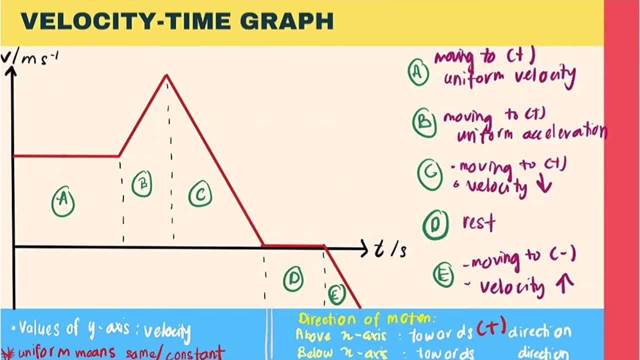 just like at E. here, this means that the object is moving towards the negative direction. At section E, the value of y-axis is negative, which indicates it is negative, and at section D the slag is negative, So the value of y-axis is negative. This means that the value is. 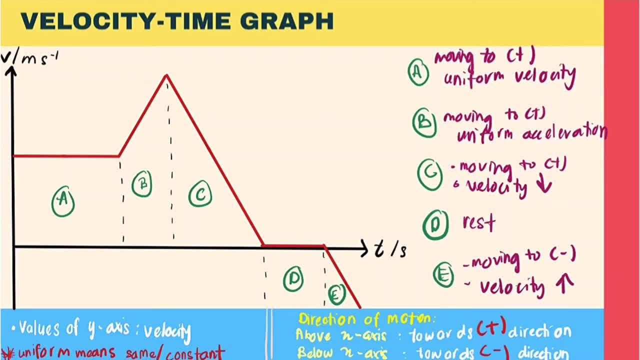 moving towards the negative direction. However, the velocity increases because as we go down the y-axis, the numbers keep on increasing from negative 1 to negative, 2 to negative 3.. Therefore, the velocity still increases, despite its negative value. I would say the positive or negative value of y-axis does not. 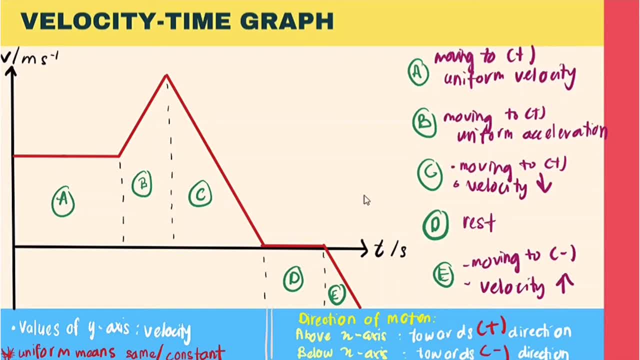 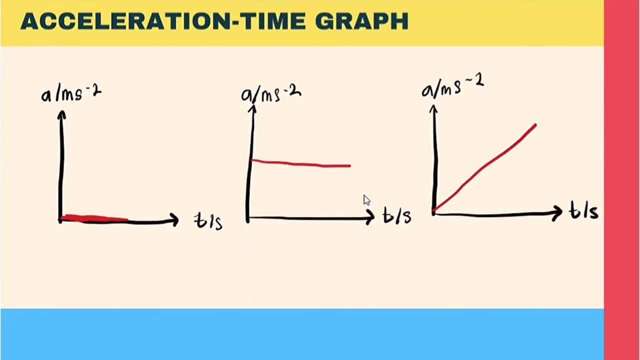 affect the velocity, but rather it's the number at the y-axis that would indicate the velocity. Finally, we have the acceleration time graph. Acceleration time graph records the acceleration at y-axis against time at the x-axis. Let's look at some basic trends of an acceleration time graph. If 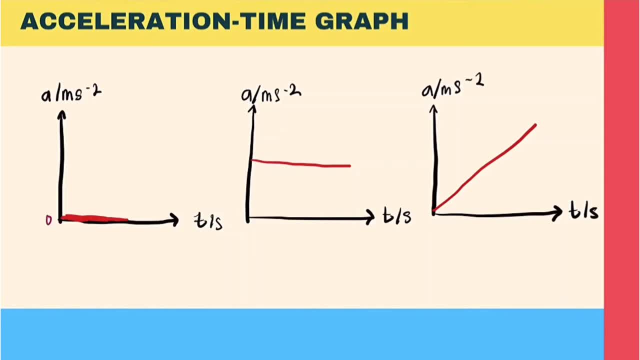 the graph is plotted straight across at 0.0 here, just like number one, this means that the object has zero acceleration. If the graph is plotted straight across at a non-zero value, just like number 2 here, this means that the object experiences a. 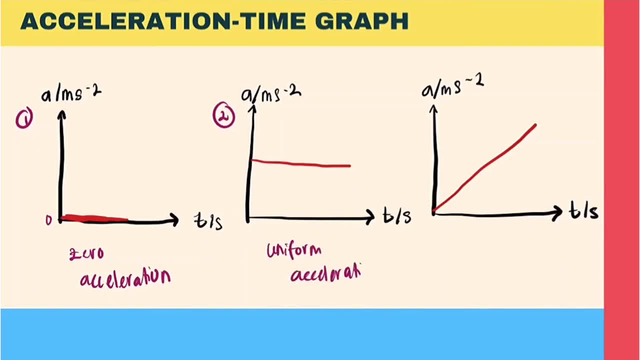 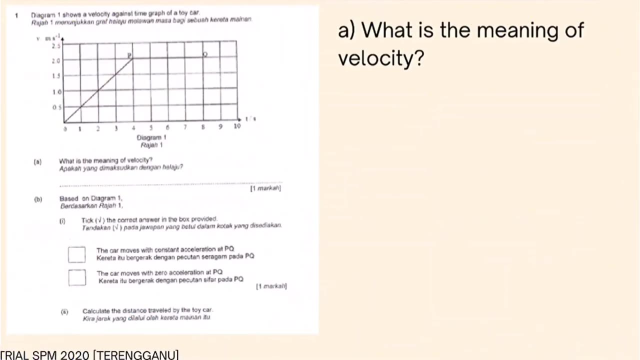 uniform acceleration. If the graph is plotted increasingly linearly, just like number 3 here, this means that the object has an increasing acceleration. Now let's answer a question together. The diagram shows a velocity against time graph of a toy car. The first question asks: what is the meaning of velocity? Velocity is the 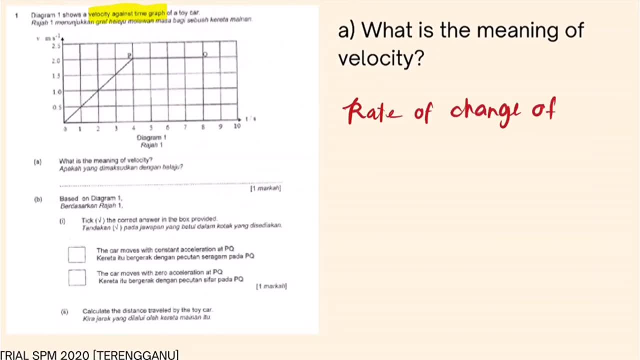 rate of change of displacement, and the keyword for the answer here is the word displacement. This will be the one that will give you the mark. The next question asks based on diagram 1,. take the correct answer in the box provided: The first. 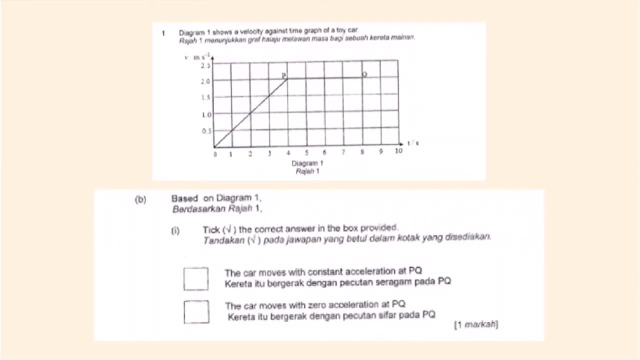 statement says the car moves with constant acceleration at PQ and the second statement says the car moves with zero acceleration at PQ. Since this is a velocity against time graph, at PQ the graph is plotted straight across, Therefore, which means at PQ it is. 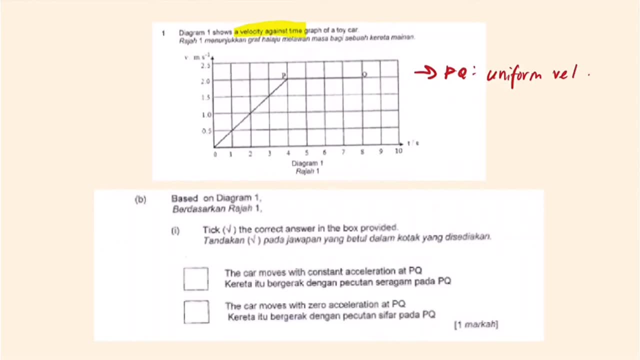 moving at uniform velocity. If an object is moving at uniform velocity, this only means that the object has no acceleration or zero acceleration. So the correct answer would be: second statement: If the car is moving with constant acceleration, then the graph should: 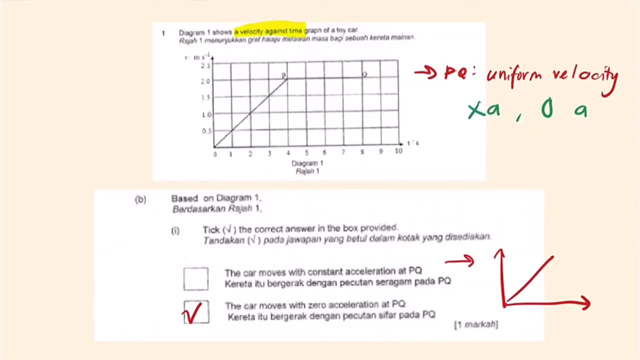 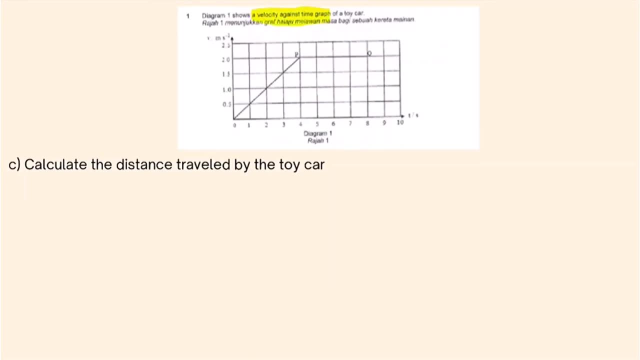 be plotted, increasing linearly, something like this: Next, the question asks us to calculate the distance travelled by the toy car. Since this is a velocity against time graph, to find the distance travelled we must find the area under the graph. So, from point O, 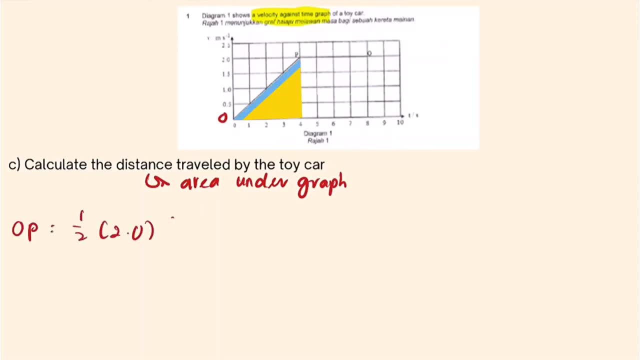 to P area under the graph would be 4.0 metres And from point B to Q, the area under the graph would be 8.0 metres, So the total distance travelled would be 4.0 metres plus 8.0 metres, which.